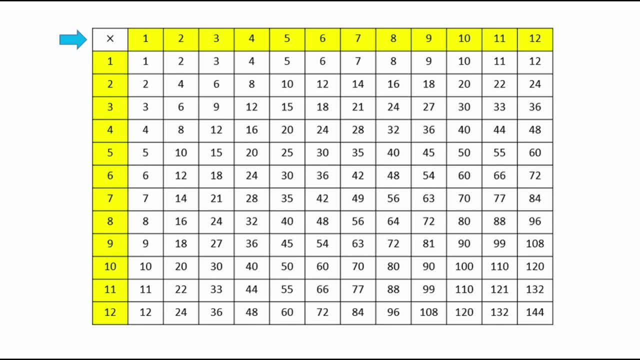 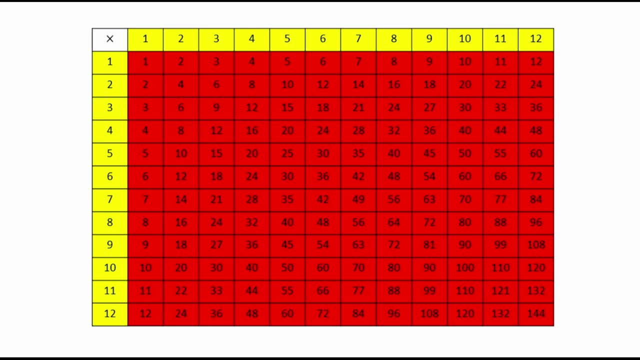 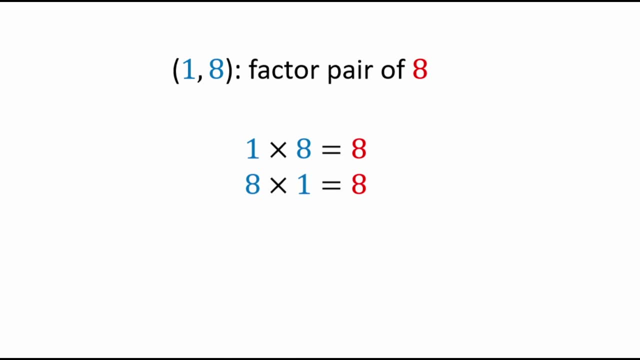 The factors that make the factor pairs are listed on the side of the table and at the top, And the products of the factor pairs are shown in the middle of the table. Let's show students how to find the factor pair or pairs that make the product of eight. 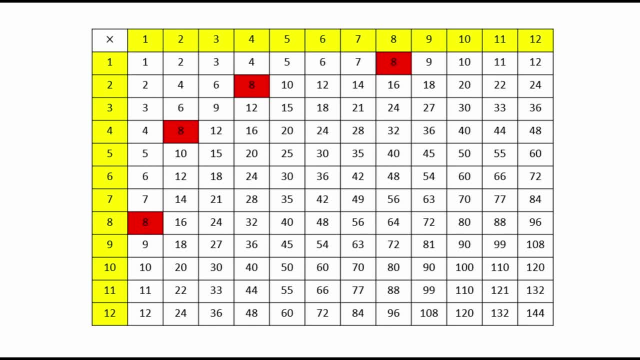 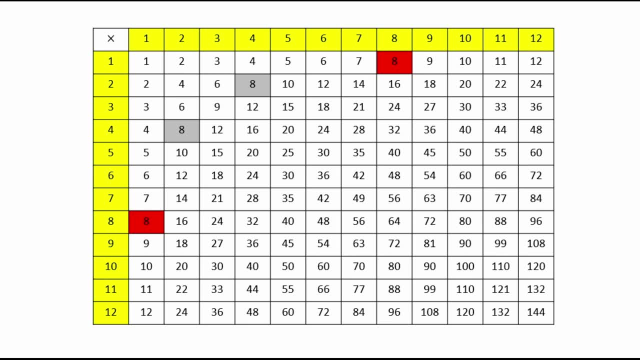 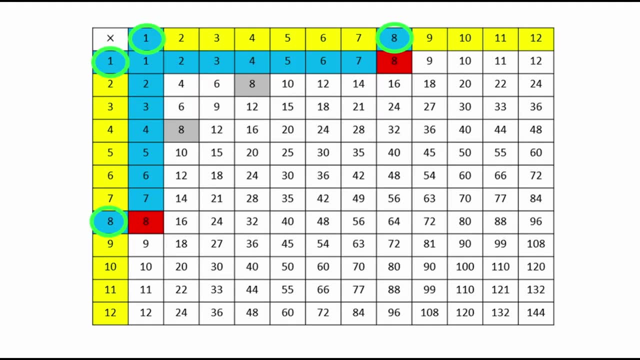 Point out to students. there are four eights shown in the middle of the table. First, have students focus on these two eights To find the two whole numbers factors that make eight. have them look at the factors in the rows and columns that intersect at eight. 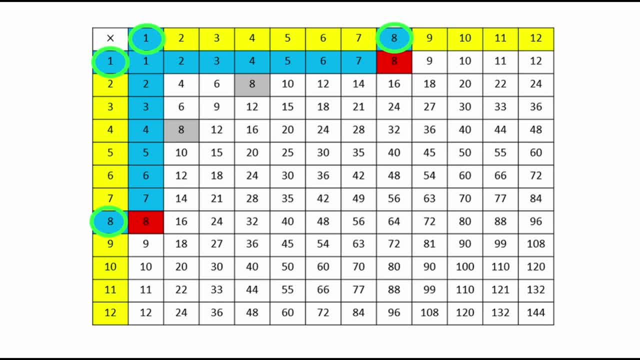 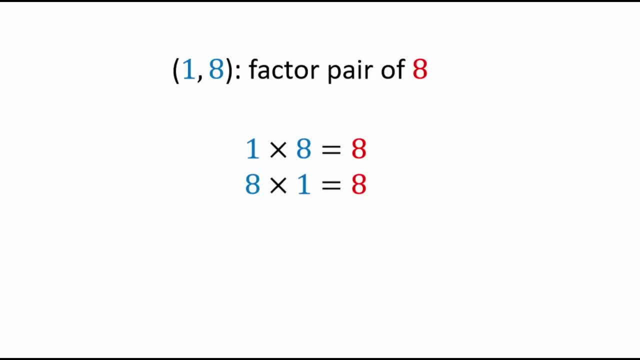 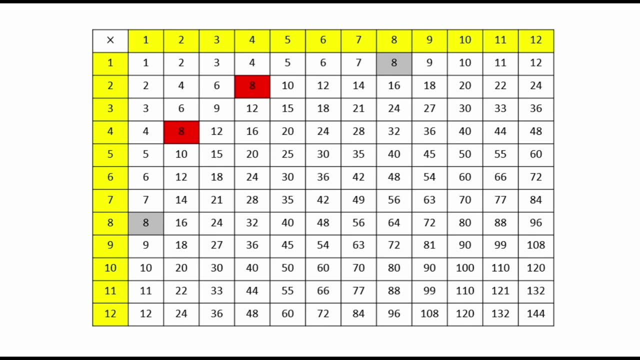 Discuss with students that the product of eight is made by the same two factors, one and eight. Tell them the numbers one and eight make a factor pair of the product of eight. Next, have students focus on the two remaining eights. Have them look at the factors in the rows and columns that intersect at eight. 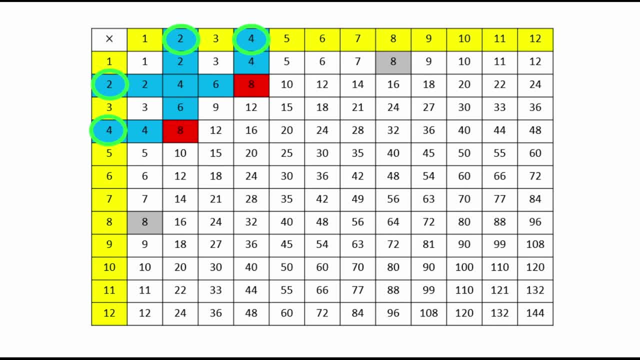 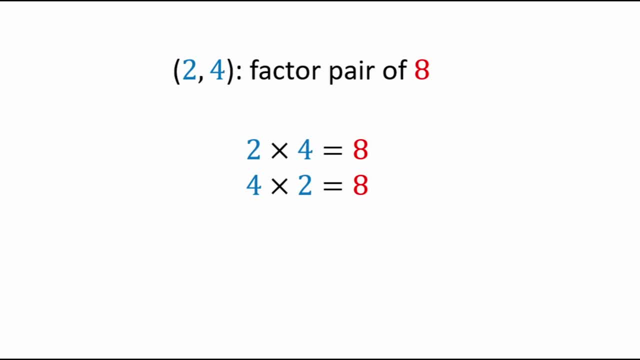 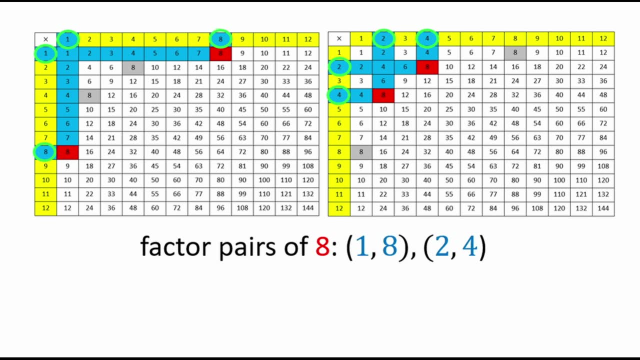 Discuss that the factors that make these two eights are the same: two and four. Tell students the numbers two and four make another factor pair of the product of eight. Last, verify that students understand the product of eight has two factor pairs: one and eight and two and four.